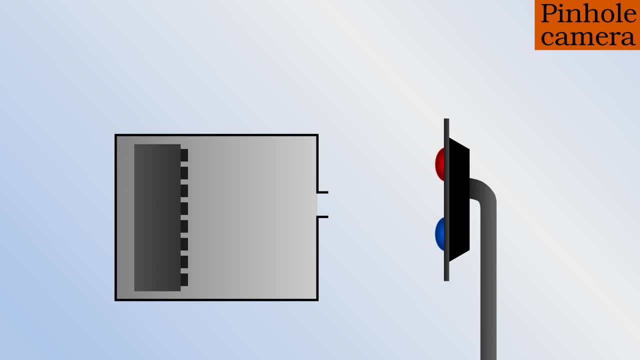 The simplest solution to this problem is to put a box around Alice's detector to block out stray light and put just a tiny hole, often called a pinhole, in front of the detector. The pinhole blocks out all but one of the red and one of the blue rays of light, so that they fall on different. 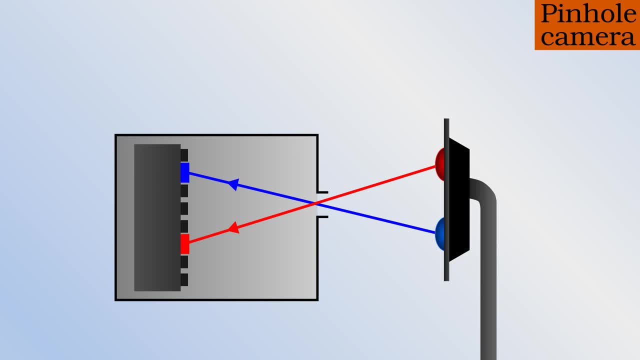 parts of the detector. The bulbs are separated in the image, which is exactly what we wanted. The image has become inverted because light from the bottom blue bulb has gone to the top and vice versa. But that's okay. this actually happens with most optics. 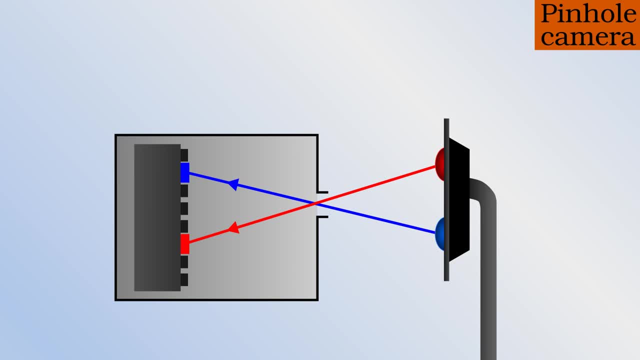 We can always use the computer to invert it back or wire up the detector to take account of this inversion. Your brain has naturally adapted to compensate for this effect in your eyes. We can always use the computer to invert it back or wire up the detector to take account of this inversion. Your brain has naturally adapted to compensate for this effect in your eyes. 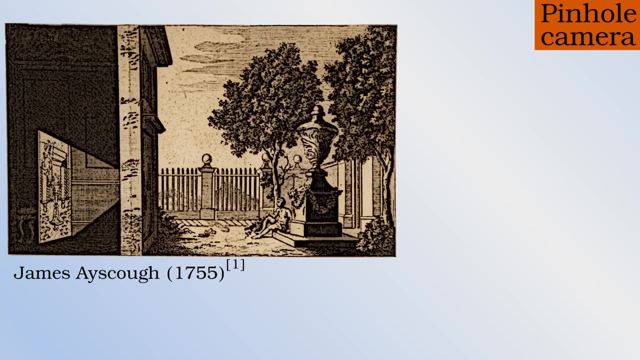 This type of darkened box with a pinhole is one of the first optical tools to be used to actually record images. The modern word camera comes from the Latin phrase camera obscura or dark chamber. Here is an 18th century illustration of a camera obscura with a pinhole. 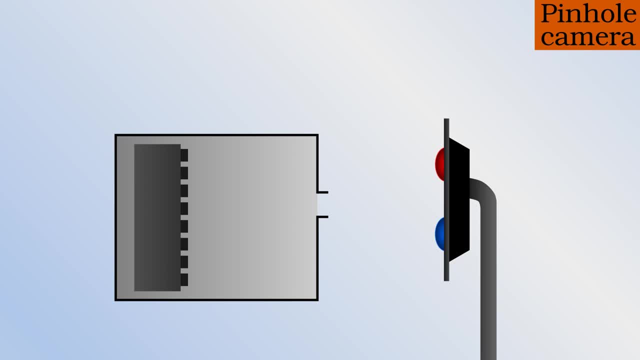 The pinhole camera illustrates the two main properties every optic must have. If the pinhole is large, too many rays get in from each of the bulbs and eventually it is as if we are back at the start, with no optic at all. If we make the pinhole smaller and smaller, 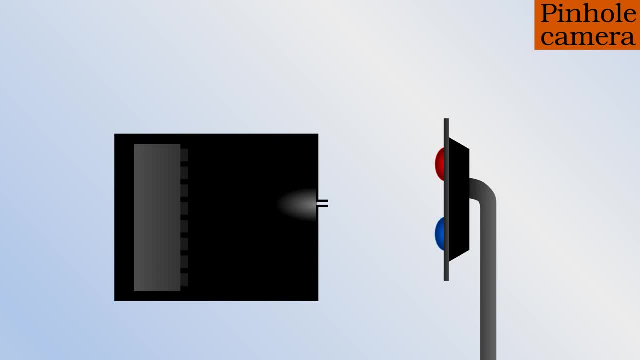 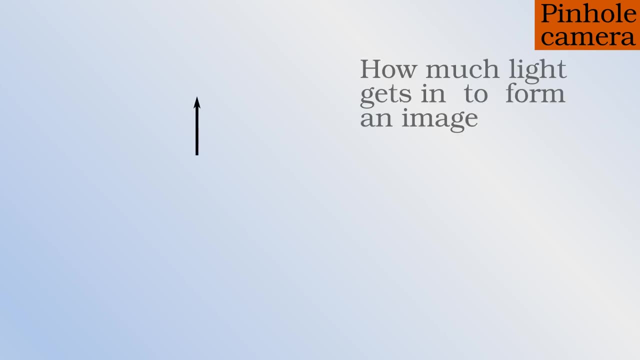 the amount of light getting in decreases and the image will become darker until it fades completely. The problem with a pinhole camera, therefore, is that it is a trade-off between how much light gets the detector to actually create the image often referred to as the size of an optic's. 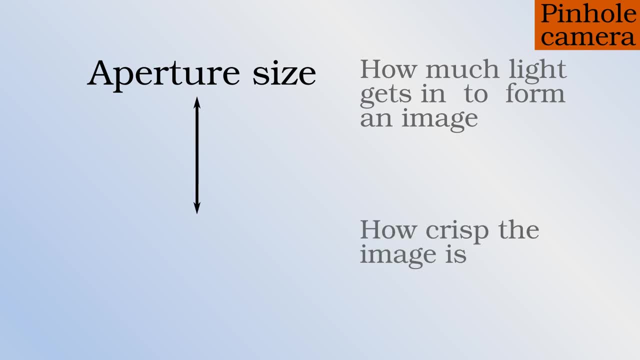 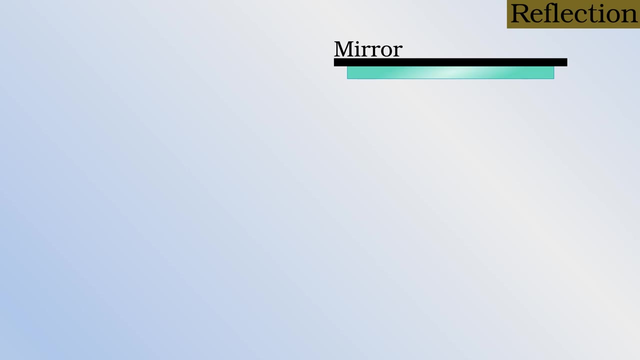 aperture and the degree to which the direction of the rays is restricted. This is the resolution of the optic which I will mention later. I don't think it is a trade-off. Ideally, we would want plenty of both. Other optics consist of mirrors which reflect the sources of light onto the detector. 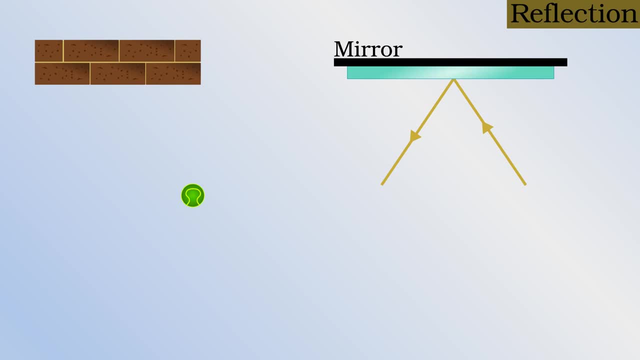 With a plain mirror, as you might have in your bathroom. light reflects the same way as a ball bouncing off a wall in the game of squash. How a ray of light is reflected depends on its direction, with the angle of incidence equal to the angle of reflection relative to a line pointing out. 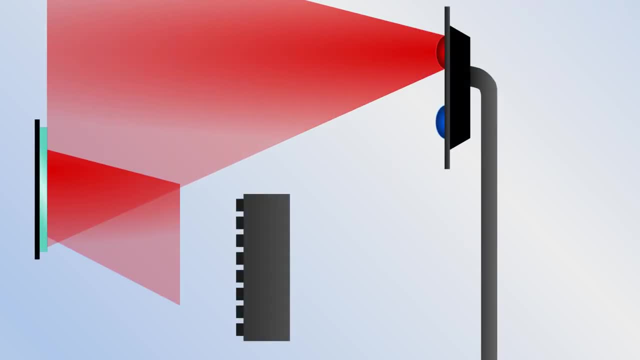 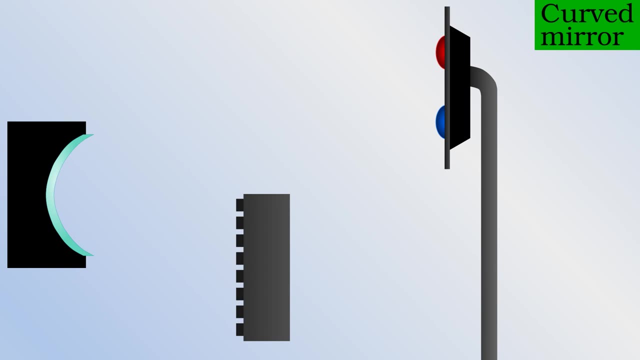 of the mirror called the normal. On its own, a plain mirror won't help us avoid the problem of the two light coming from the detector and the whole detector purple we saw earlier. Instead, the mirror must be curved either into a part of a sphere or into a special shape called a parabola. 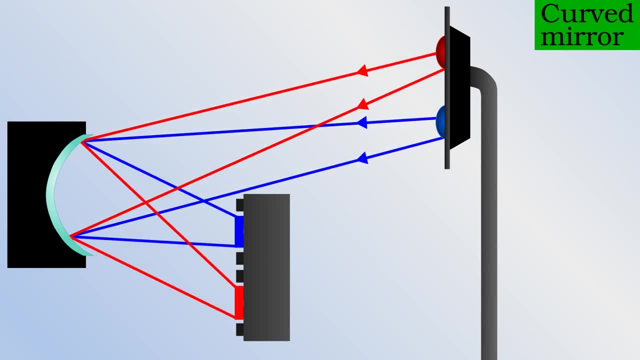 What this shape of mirror means is that when rays from the two bulbs come in, and they do so at different angles, they are reflected to different parts of the detector. In fact, all the blue rays go to one part and all the red ones to another. Just as with the pinhole, the image is inverted. 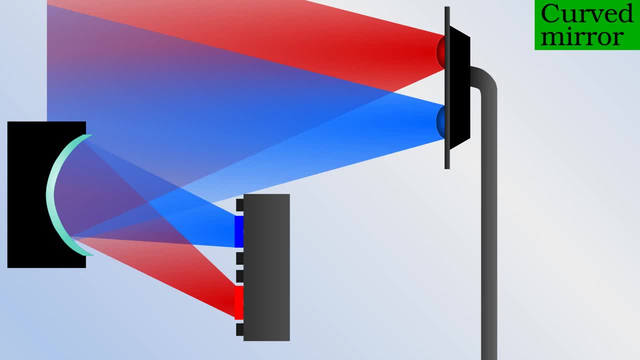 but light from the two bulbs goes to separate parts of the detector as required. setup solves the main problem of the pinhole, because you can make the mirror as large as you like in principle, and therefore collect plenty of light while still forming a clear image. However, 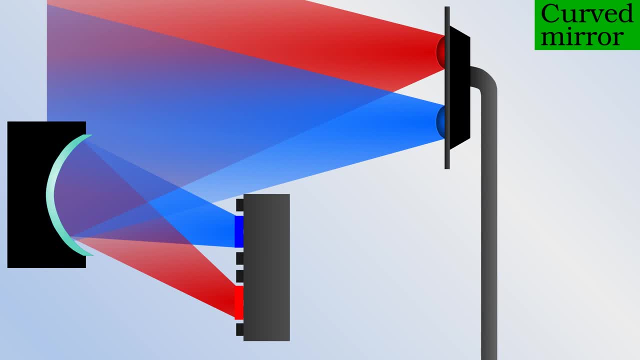 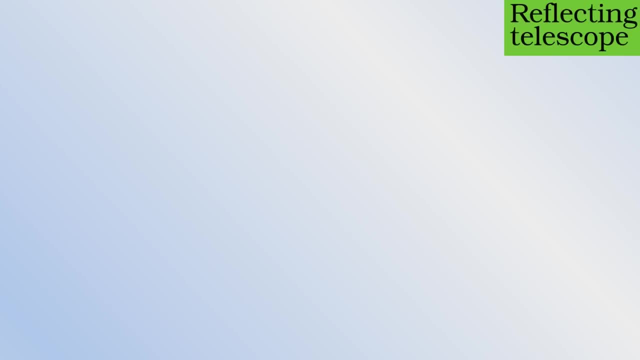 the main disadvantage of this type of optic is that it's cumbersome and very long, due in part to the light being reflected back on itself. For this reason, this setup is mainly used for telescopes. The telescope tube forms the dark chamber to block out stray light and usually a 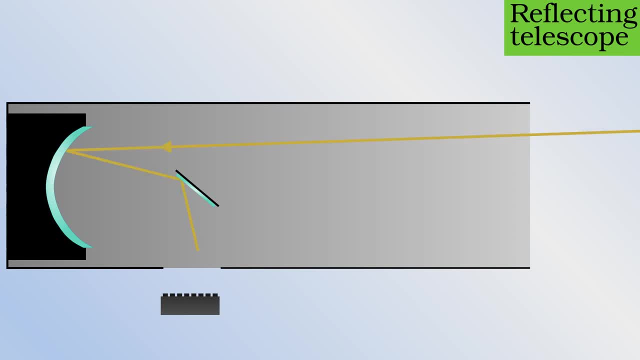 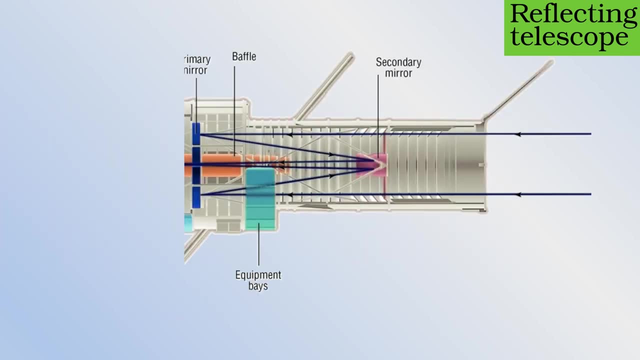 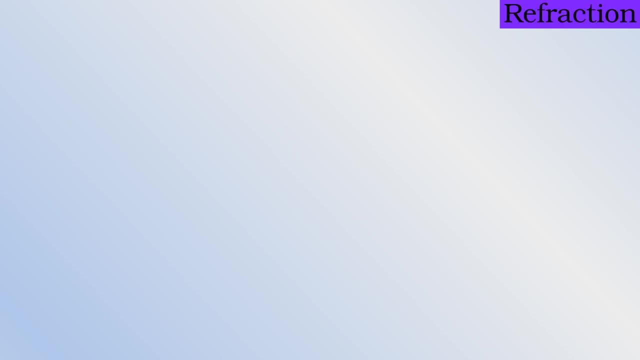 second plane mirror is added just to divert away the light to the detector. The first known working mirror telescope was made by Isaac Newton, and more recently the Hubble Space Telescope used a similar but slightly more complicated arrangement. This brings me on to lenses, a type of optic which 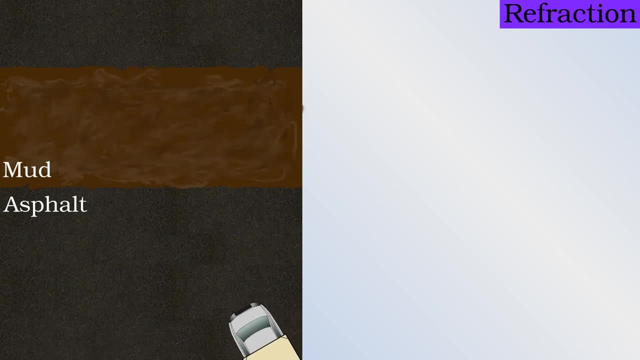 uses refraction. Imagine that you have a truck running on a hard road and suddenly it hits the edge of a muddy field at an angle For a moment. only one of its tires is on the mud. so one side of the tire is on the mud, The other side is on the mud. The other side is on the mud. 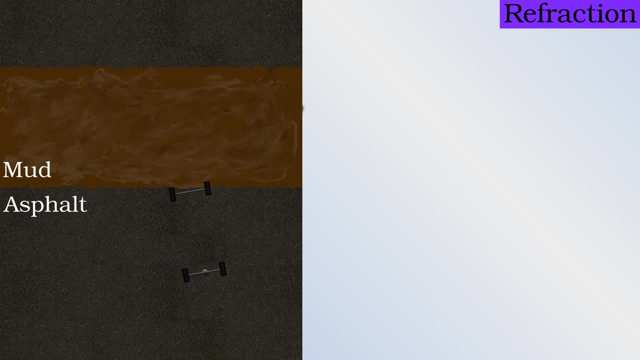 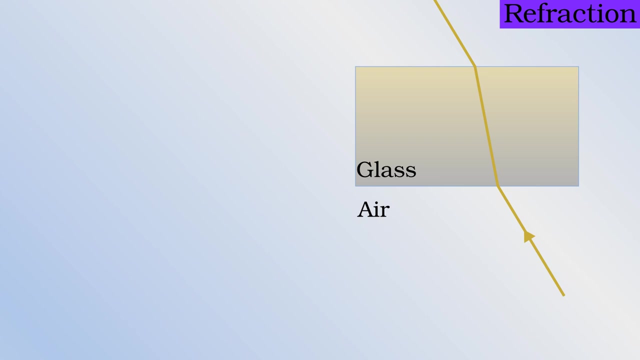 The other side of the truck slows down while the other continues at speed. The truck turns In a similar way, light bends or refracts into a dense material like glass and refracts in the opposite direction. when it transitions from glass to air With a rectangular glass block, the light enters. 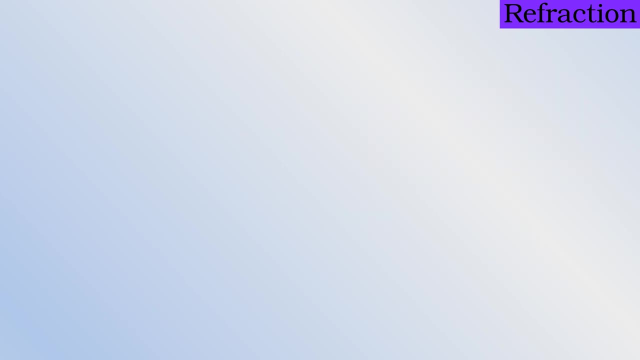 and leaves going in the same direction. just shifted slightly, Having the two opposite sides inclined alters the direction of the emerging ray in proportion to the slanting. By curving the shape of the glass, it's able to go in the same direction. The light enters and leaves going in the same. 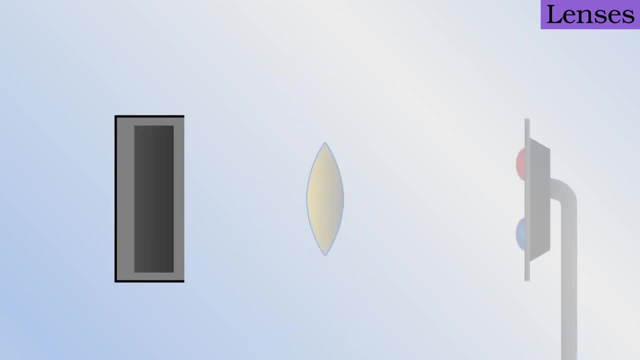 direction. By curving the shape of the glass, it's able to go in the same direction. By curving the shape of the glass, it's able to go in the same direction. The light enters and leaves, going in the same direction, In a similar manner to the curved mirror from before. rays of red and blue light will likewise. 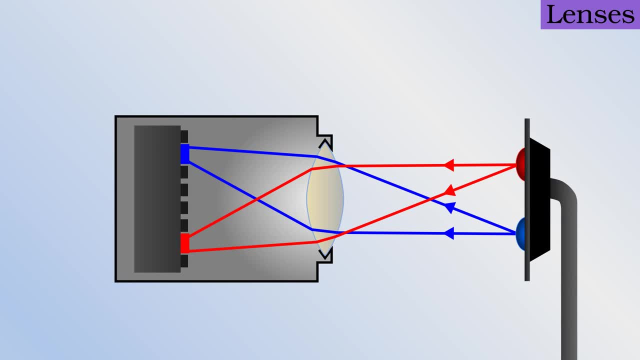 be diverted to different parts of the detector. Just like with the mirror, a lens can be made larger to emit more light while still maintaining a crisp image. The advantage of the lens is that it allows a practical and compact optical device such as the human eye or a cell phone camera. 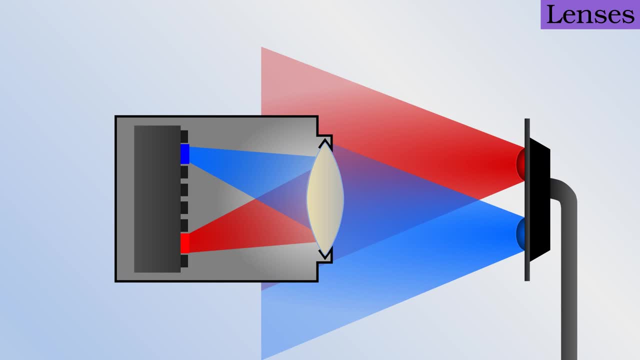 The lens is at the front to focus light, there is a chamber to block any stray light and the detector is at the back. The lens is at the front to focus light, there is a chamber to block any stray light and the detector is at the back. This makes the lens into the most ubiquitous. 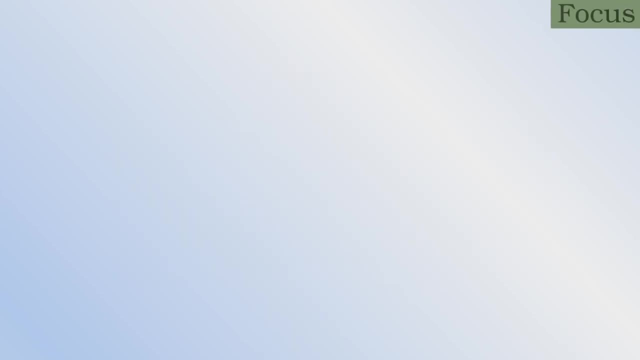 and important type of optic. Usually a high level optics textbook or a class would talk about what happens to a single point of light. They talk about things like the point spread function of an optic, the pattern of light that a point source produces on a detector. This is because we can. 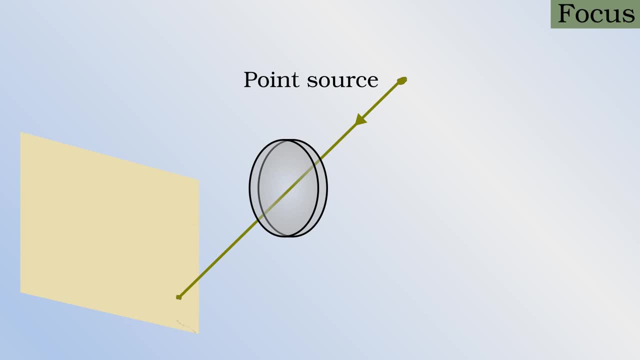 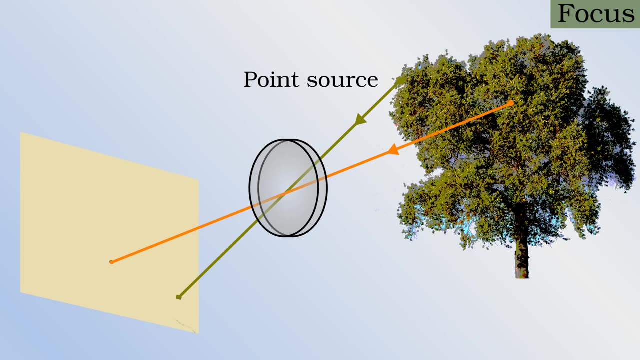 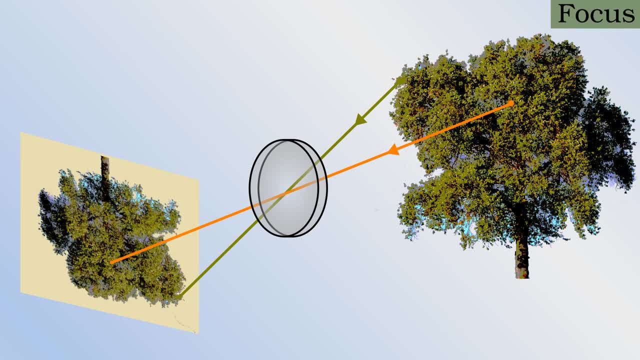 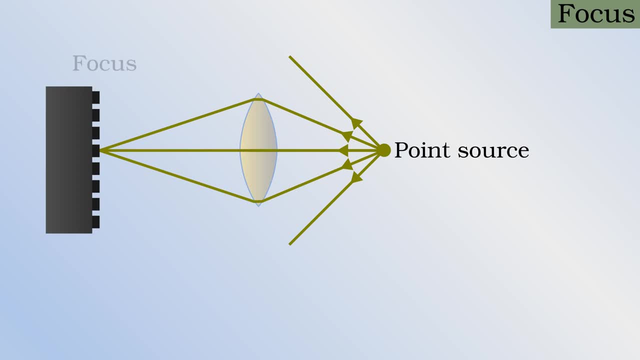 source in all directions and to redirect them, using reflection refraction or other ways I haven't mentioned- to a single pixel on our detector. I will talk only about lenses from now on, but the same arguments apply to other optics like the Newtonian telescope I mentioned. 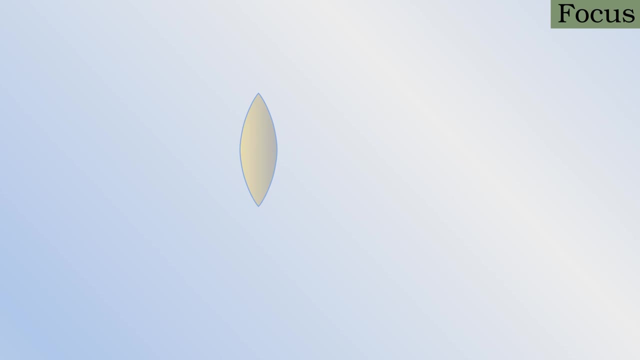 Based upon their shape and other properties, every lens has a so-called focal length. When the point source you are observing is very far away, almost infinitely far away in fact, then this is the precise distance behind the lens that the rays converge and the light is focused. This is therefore the precise distance at which to place the detector. 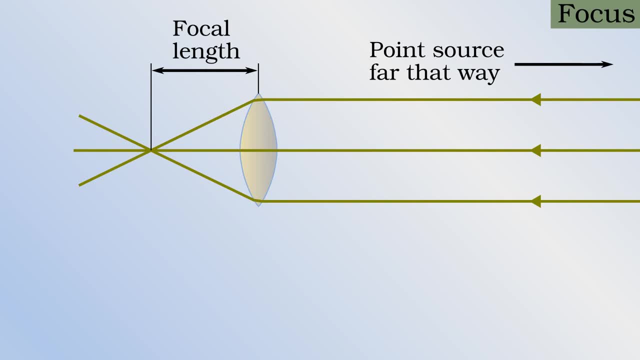 behind the lens. If you put the detector too close, then the rays of light haven't yet converged on a single point. If you put the detector too far from the lens, the rays have begun to diverge again. Both cases show what it would be like to have a light source that is so close to the detector. but 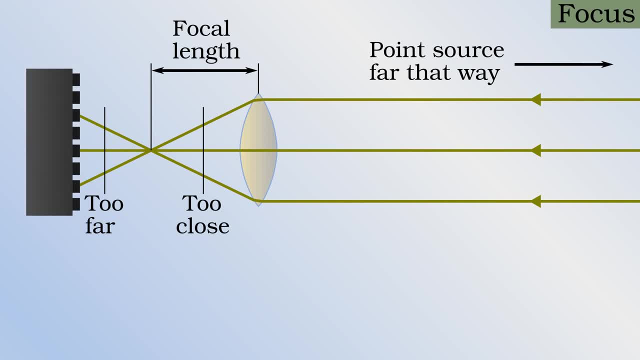 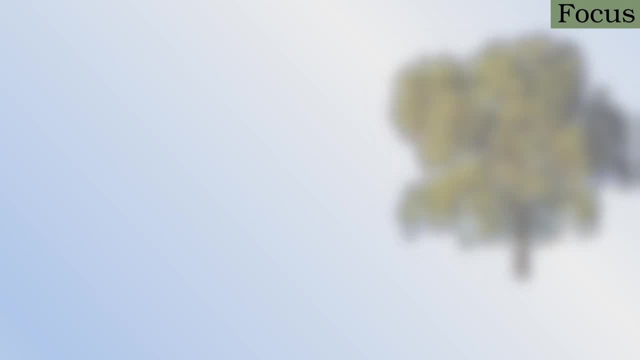 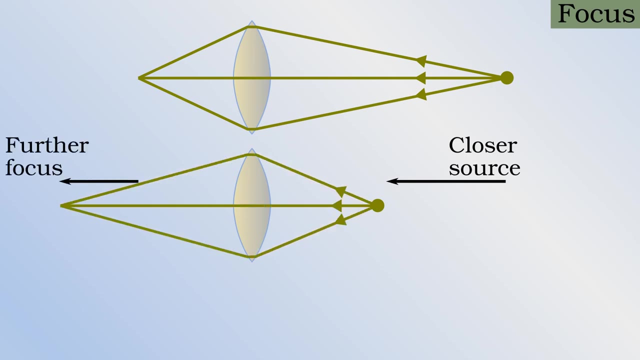 what it means to be out of focus. Each point of light now spills over multiple pixels and the whole image becomes blurry, as you can simulate with the blur tool in many image editing programs. The closer the point source comes to the lens, the further the focus moves behind the lens. 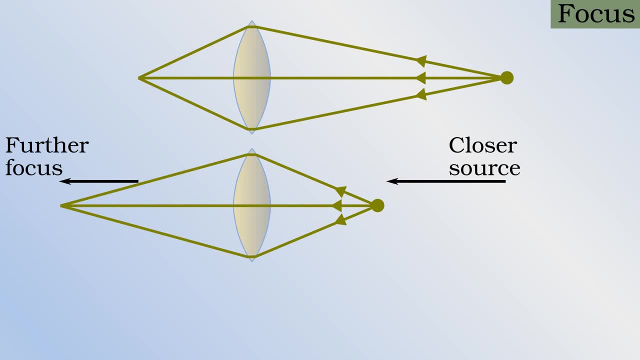 There is a precise mathematical relationship between the focal length, the distance from the object to the lens and the distance to the resulting focus. This shifting of the focus is a problem if you have just set up a lens with the focus, If you have set up your detector exactly one focal length behind the lens to image things in the far distance and now want to image a closer object. 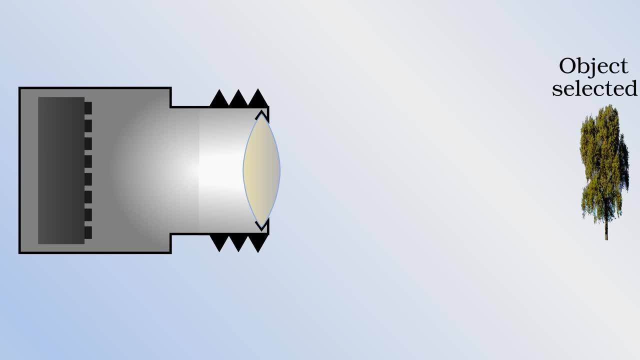 cameras and eyes overcome this issue in two particular ways. when taking a photograph with a camera, once the object to be focused on has been selected, the lens will be moved by the photographer or automatically by the internal circuitry of the camera to pick the right distance between it and the detector. 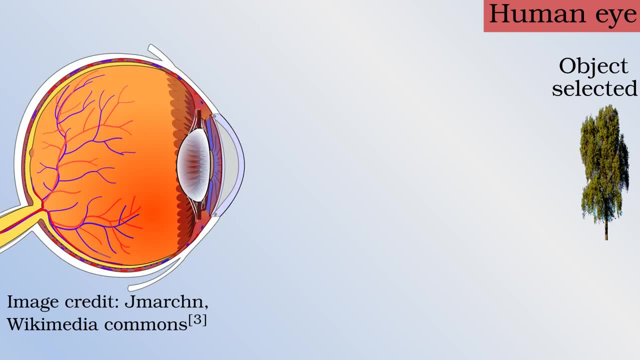 The size of the human eye is fixed, so instead muscles change the focus shape of the lens and therefore its focal length, to shift the focus backwards or forwards as required. In this way, the light sensitive cells in a layer called the retina, which is the detector, 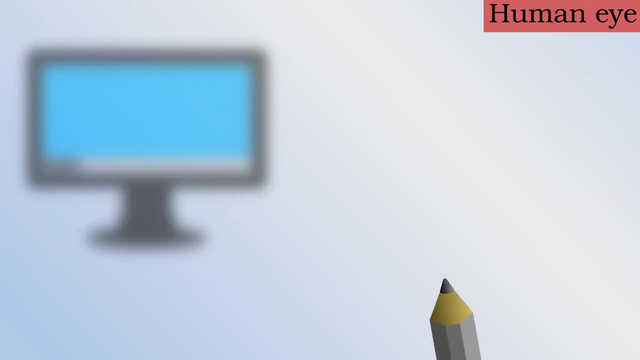 in your eye can stay where they are. Try to hold a pencil close to your face. You can either choose to focus on the pencil, in which case the background goes blurry, or vice versa. Either way, your brain is automatically using muscles to stretch or compress the lens in. 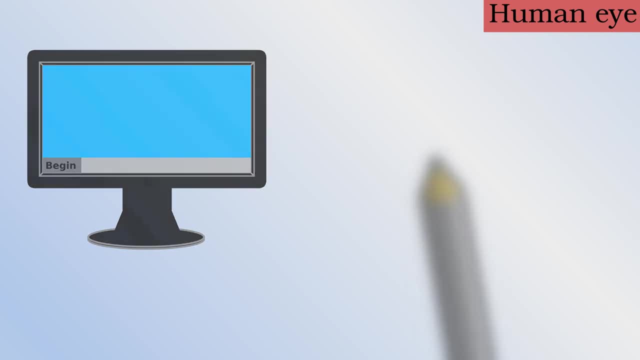 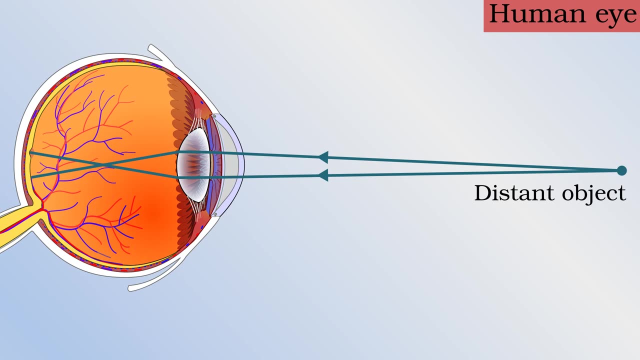 your eye to achieve the correct focal length to focus on what you want. As I've just explained, if an object is far away, then light is focused close to the lens. For some people, no matter how much their muscles try to adjust the lens, they can never. 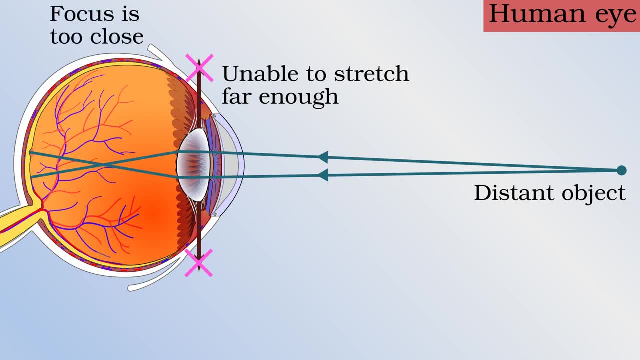 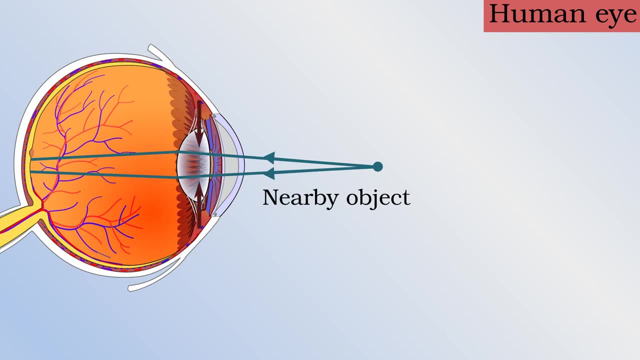 shift the focus of a distant object backwards far enough onto the retina, and they are near-sighted. Conversely, when objects are close, some people can never quite manage to shift the focal point far enough forward, and they are far-sighted. Glasses or contact lenses can correct for these problems. 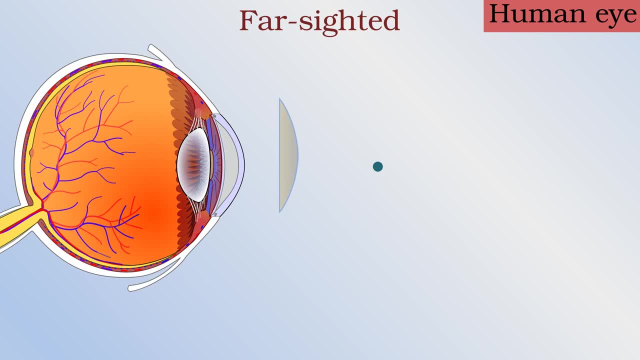 In the far-sighted example, the problem was that rays of light were diverging too strongly from a nearby object, but an additional lens can bend the rays inwards as if they were coming from a distant object. For near-sighted people, the lens makes rays diverge as if the object were closer.